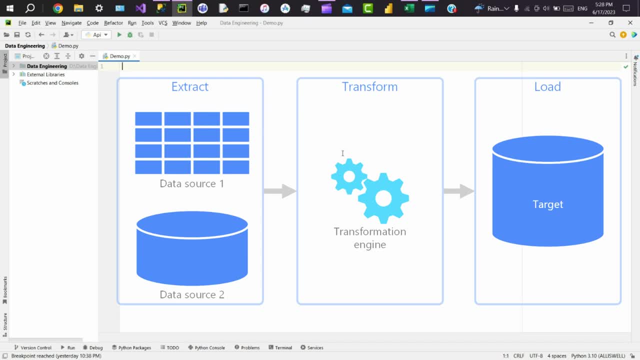 rest: apis, crms and more. Then the next step is transform, where we transform the data according to the business requirements or logic. The third step is to load the transformed data into data warehouse or target system. Now we will see how to pull data from an API using. 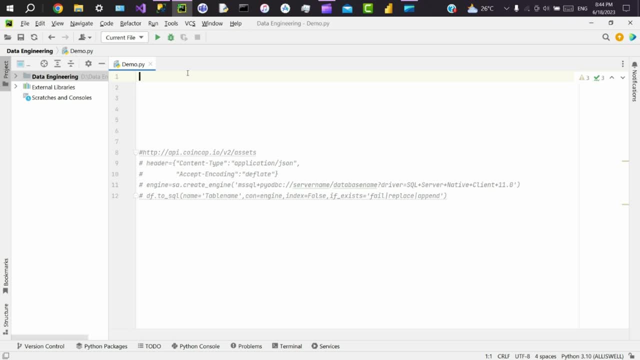 python and load it into any of the databases. So for this we need to import three packages. first, Import request. Using request package we can perform CRUD operations, that is, get, post put, delete and more. on an API, We will import pandas. This is to convert the JSON data we receive from an API to data frame. The third: 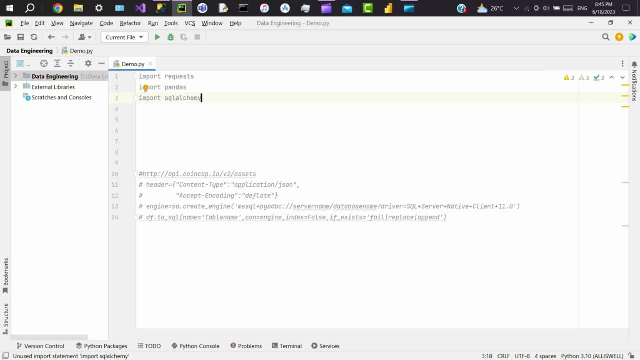 one is SQL alchemy. Using SQL alchemy, we can create a connection between database and python. So we will create a variable called url and we will assign our API link. This is an open API. This provides real-time cryptocurrency data. Now we will create a dictionary and pass all. 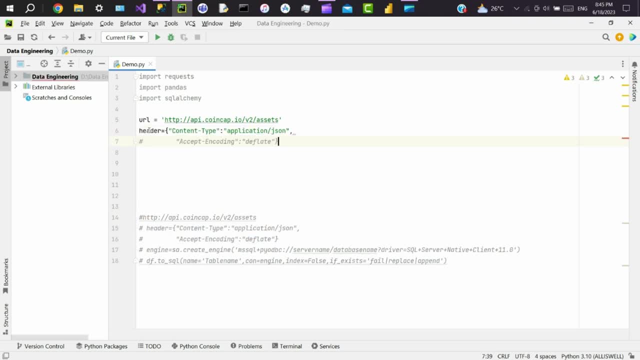 the headers required to access the API. These two are the headers we need to pass to access this API. If you are trying to pull organization data from an API, it should be authorized with an API key, So make sure to pass all the headers in the format. 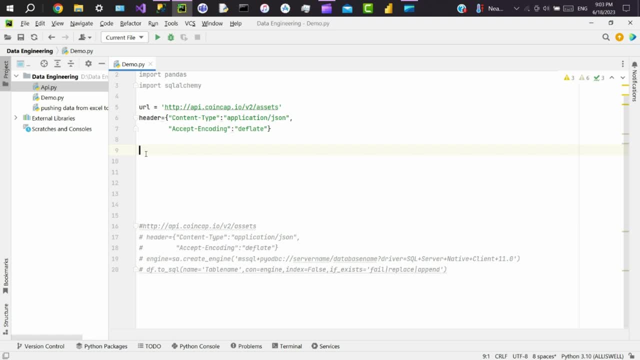 Now we will use get method to pull data: Press enter or remember to type in the URL after choosing the header and the password. here we'll use get method. We'll print the response and see. We'll create our API Resonance. 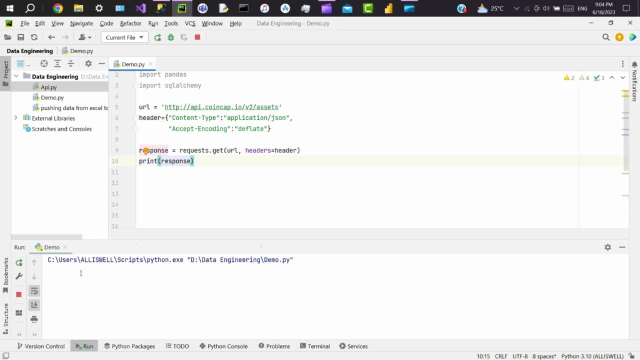 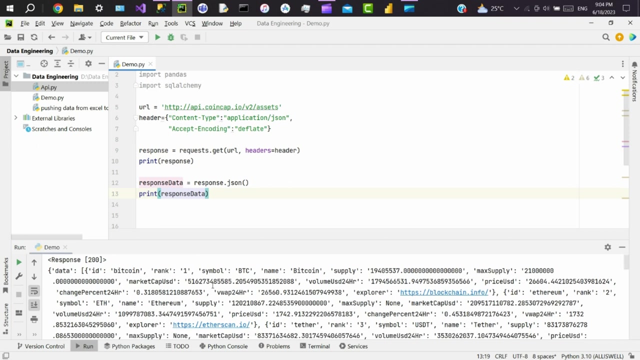 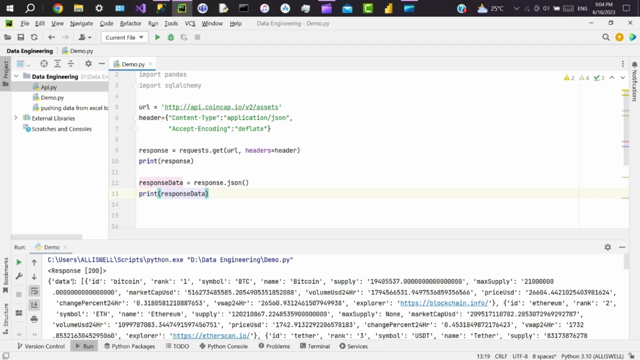 the status code is 200, which means the request has succeeded. create another variable response data to show the json data. use json method response. json json data. the api has returned cryptocurrency data. if you see, here our actual data is a value to the key data, so it is nested. we need to normalize this, so we'll use. 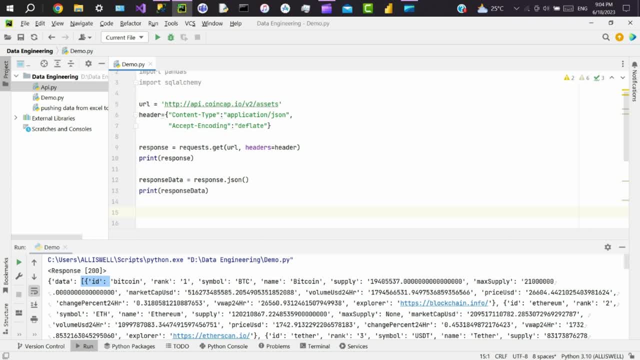 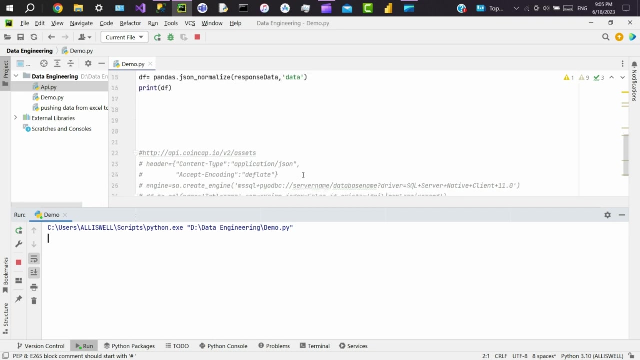 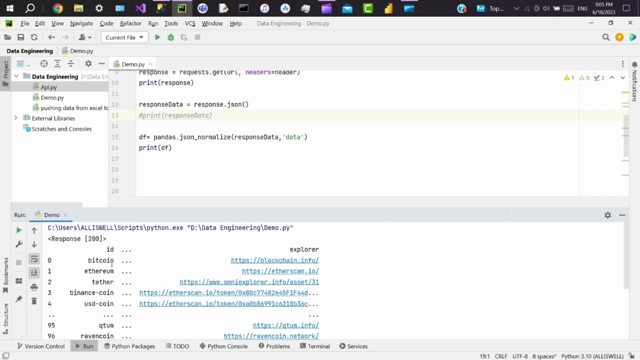 this and normalize, function with the frame equal to, and thus as response data, and pass the key which we have to normalize, that is, data, to bring the data frame. now we'll see it is in the form of rows and columns, which is data to database we have. 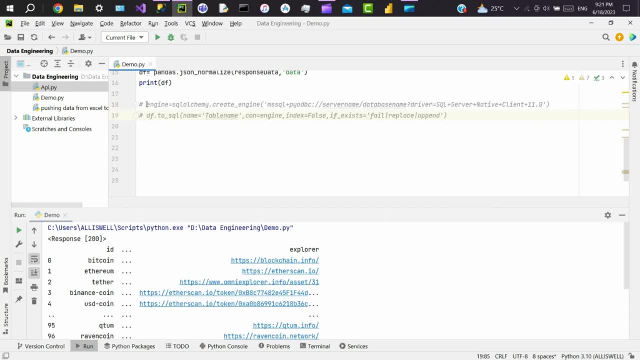 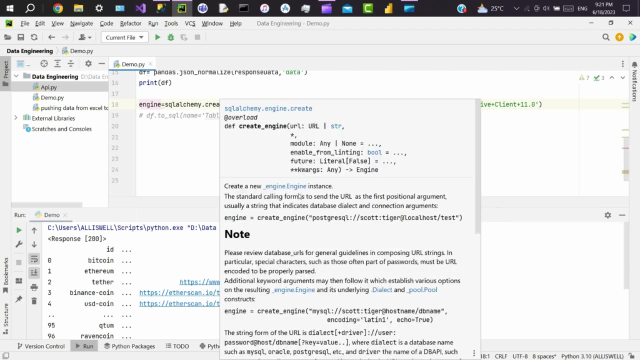 to create a connection. first here is the syntax: i'm creating a connection between microsoft sql server and python, so typing it as ms sql plus piodbc. if you want to create a connection between python and any other database, just go to the documentation of create engine. 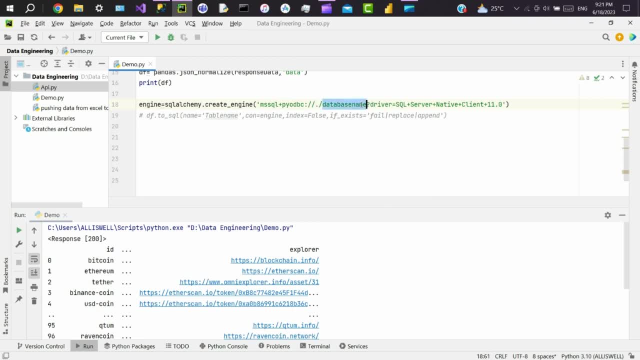 pass the server name- here i'm using local database name- and use tool sql method to push the data to the table. name it as and to the connection. pass the engine we created. if you want to load this column as well, make the index as true, if not, just put it as false. and another parameter called if. 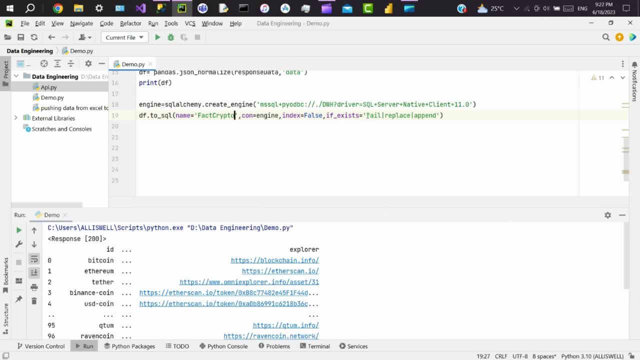 exists. we can pass three values here: fail, replace and append. if there is no table created, use. if there is already a table created with the name fact crypto and you want to replace it, use replace. if you want to do incremental load, use append. for now, i'll use fail. 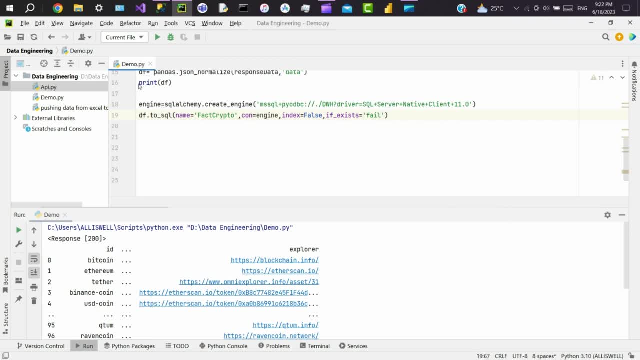 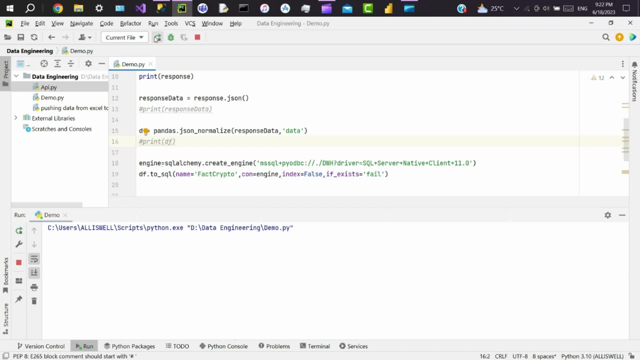 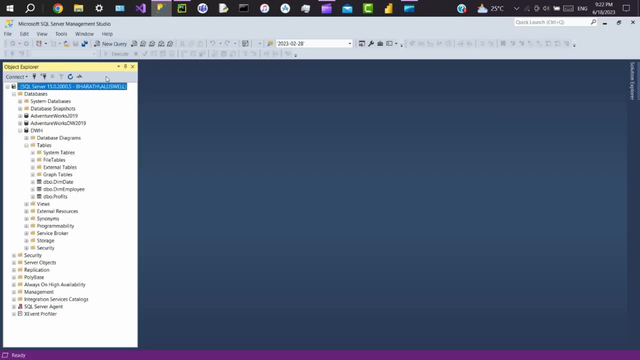 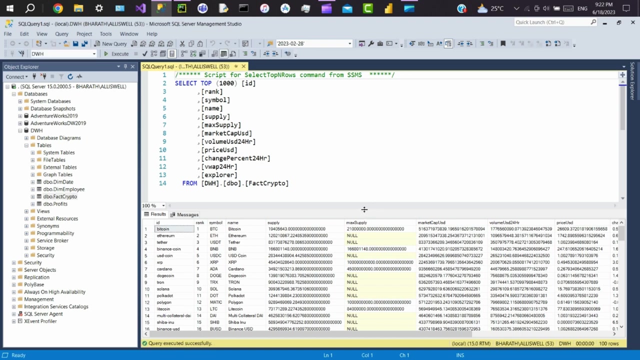 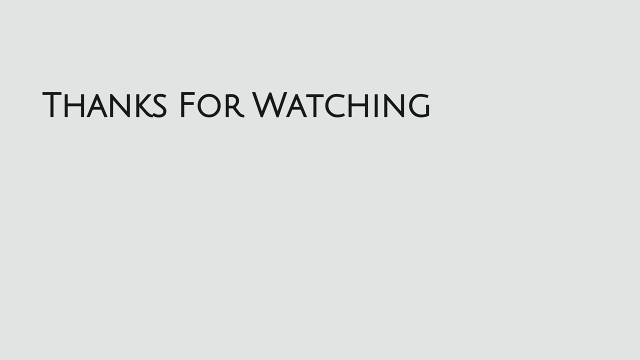 this one and execute the file. this succeeded. we'll go to our ms sql refresh the table. there's a table called fact crypto. here you can see data from api got loaded into sql server. thanks for watching you, you.